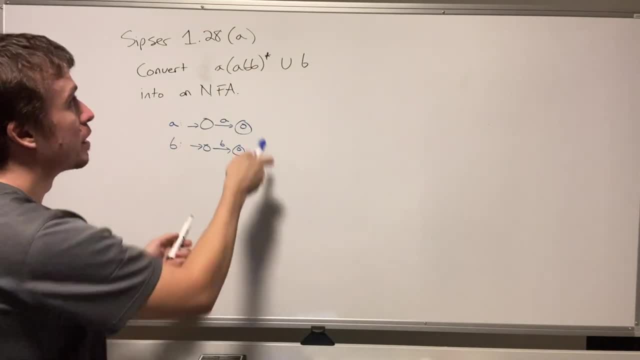 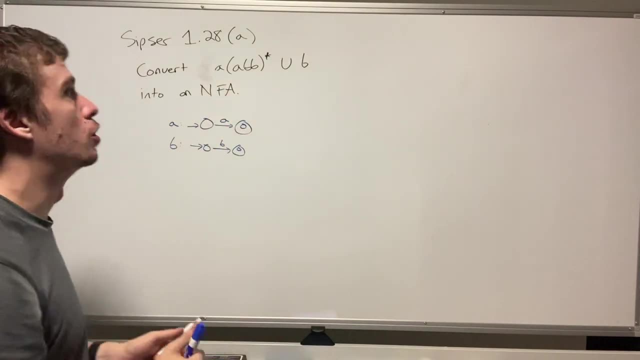 So generally you want to start with the thing on the innermost layer, and by layer here I mean within the parentheses. So if they're like parentheses within those, you want to work with those first. It's kind of like a mathematical expression with PEMDAS. 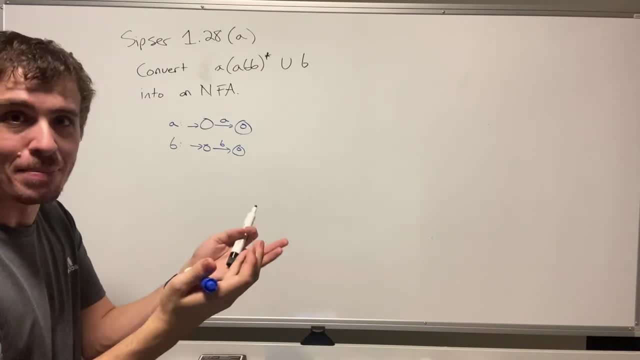 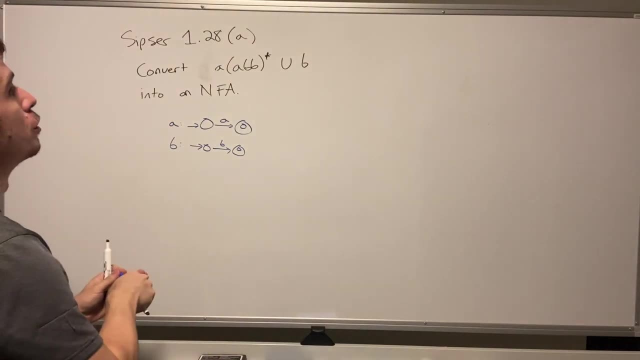 You work with the inner things, first because of the P in PEMDAS, and then you work your way out. Same idea here And there's actually an analogy there, but I'm not going to go into it. All right. so then what we can do is: let's work with two pieces, So let's do A, B And remember. 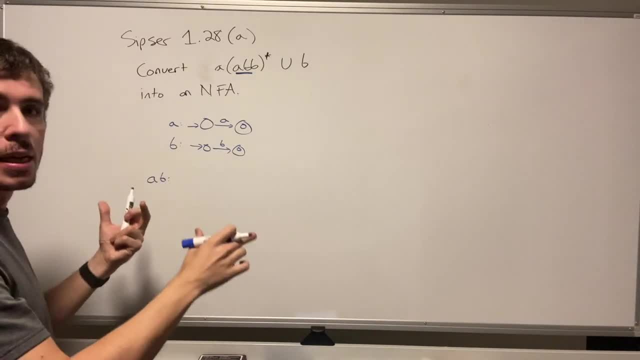 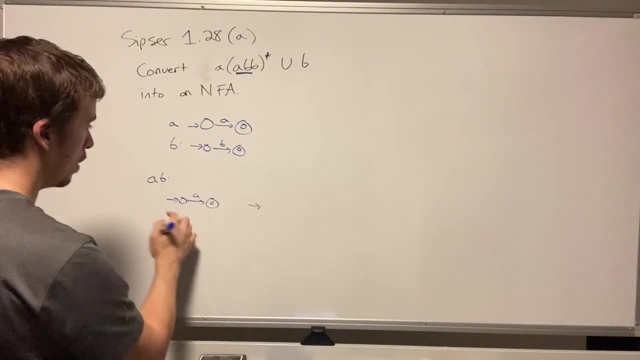 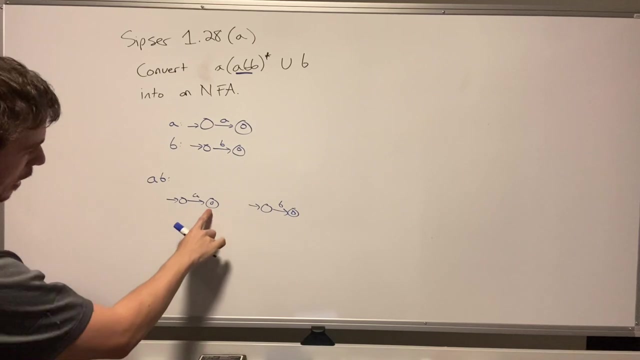 for concatenation, all we need to do is to take the two things, And so I'm going to copy and paste them down, and then we will connect one up to the other. So the A is obviously going to go first and then the B next. So then what we need to do is to connect every final state of the first side. 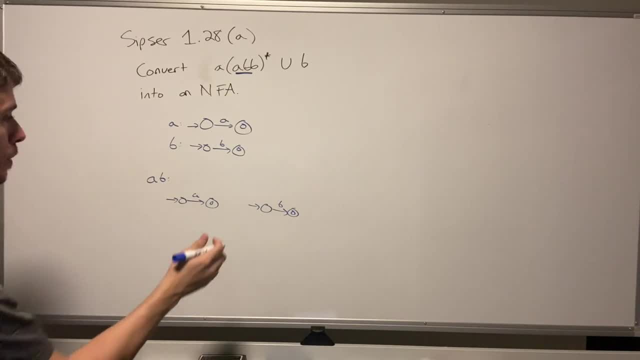 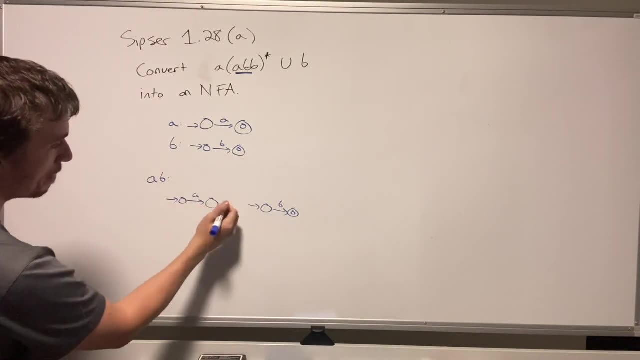 into the start state of the second side with an epsilon transition and make the the original state non-final here. So if there are multiple states here, they would all be non-final, And so we'll all have an epsilon transition to this one state here. Okay, and by the way, there is a way. 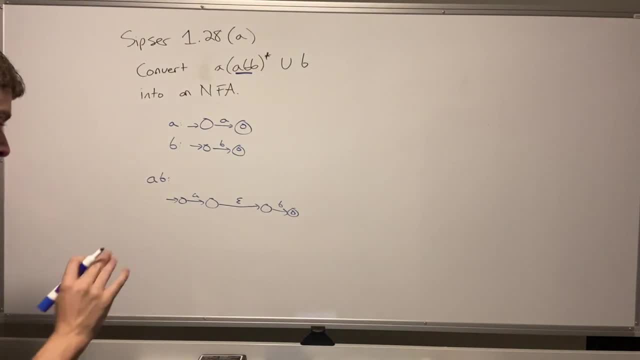 to avoid this epsilon transition, but I'm not going to go into that. So you can make a smaller NFA for this, but I want this to be an algorithmic method that always works. All right, so then for A, B, B. 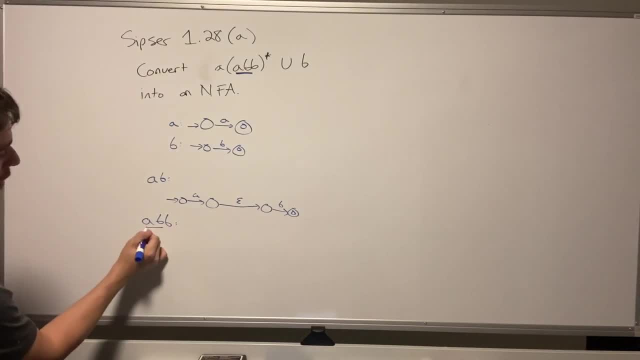 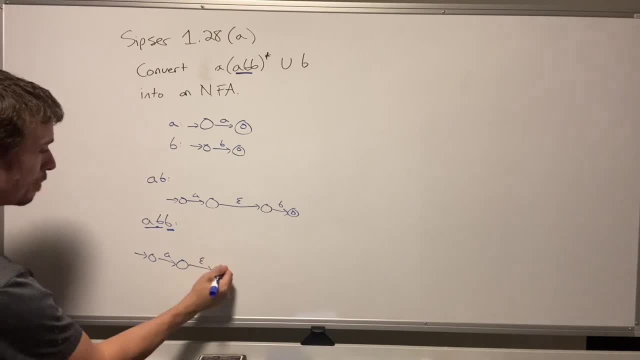 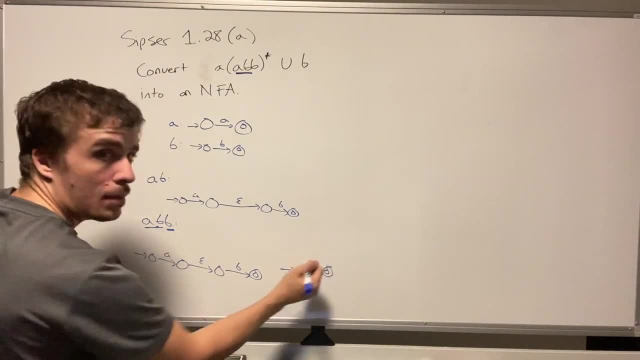 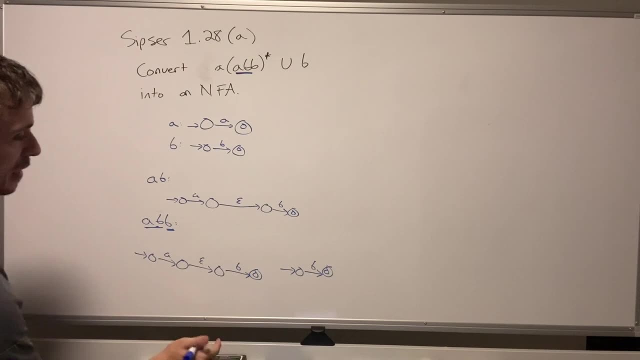 going to have a right half, Okay, and then now I'm going to again connect every final state of the first half to the start state of the second half by and making it non-final with an epsilon transition. So you can kind of see that the the pattern was going to hold anyway. 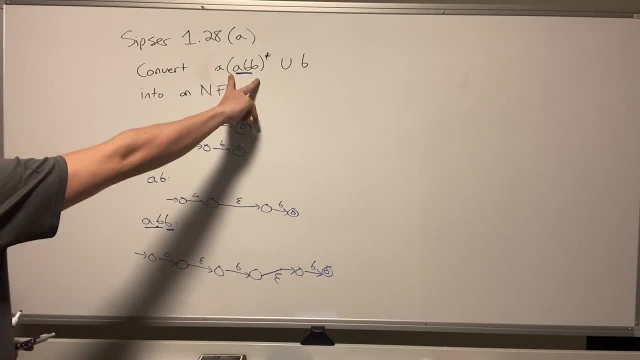 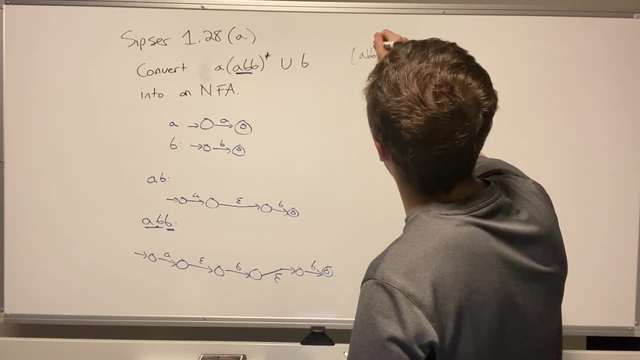 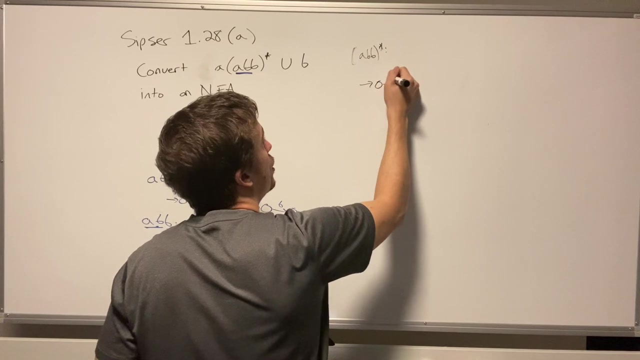 but it's just nice to see if it actually works. All right, so let's, let's take the star into account. So I'm going to change to black here: A, B, B star. So I'm going to copy and paste this thing. So I'm going to have this, So A. 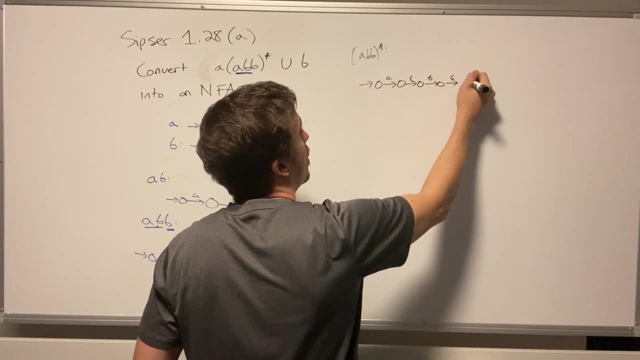 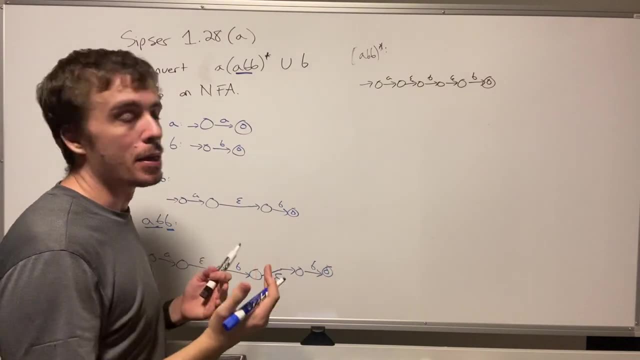 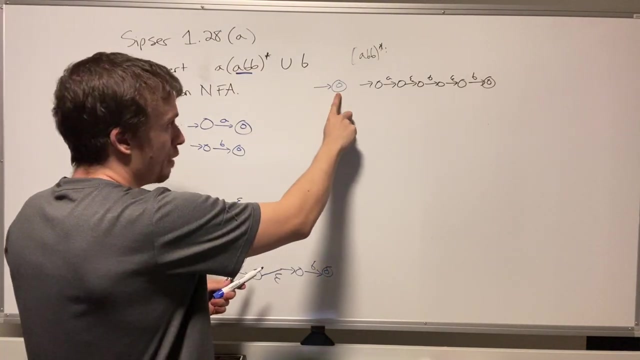 epsilon B, epsilon B, And then for the star part, what we need to do is to make a new start state- Although there is a way to actually avoid this kind of but- which is a final state, because the empty string is in the star of anything. 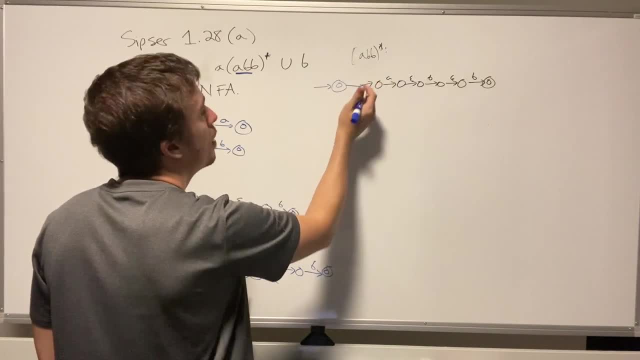 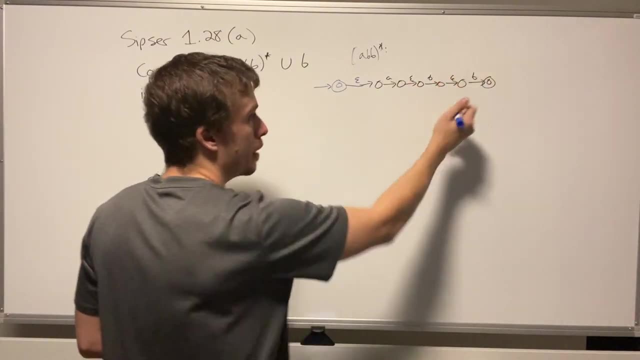 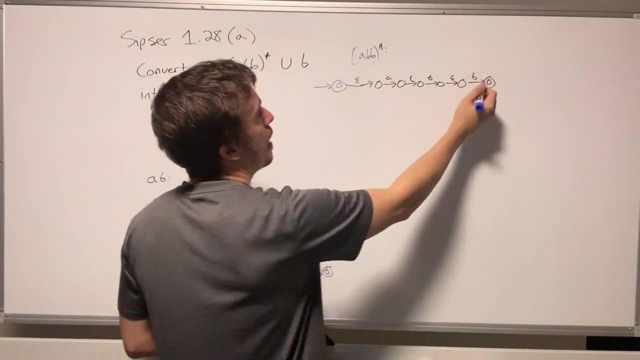 So, and what happens is we do an epsilon transition into the start state from from this brand new guy, And every pre in every final state over here will epsilon its way back to either the, the actual new star state or the old one, It doesn't actually matter, I'm going to do it to the brand new one. 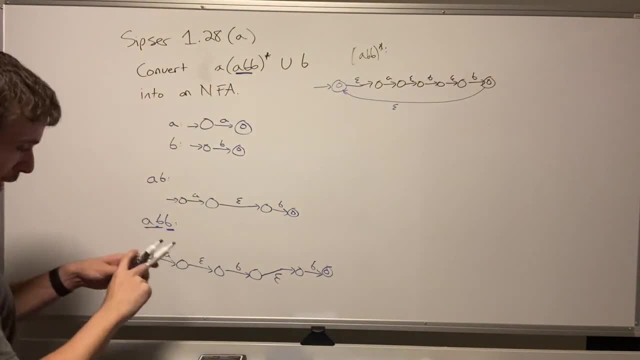 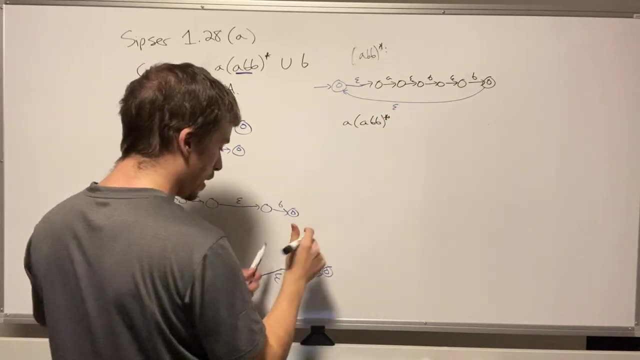 So that, that's the star now. So then now let's do the concatenation of the two. So we're going to have A, A, B, B star, And it's pretty obvious what's going to happen here. So I'm going to have the A machine. 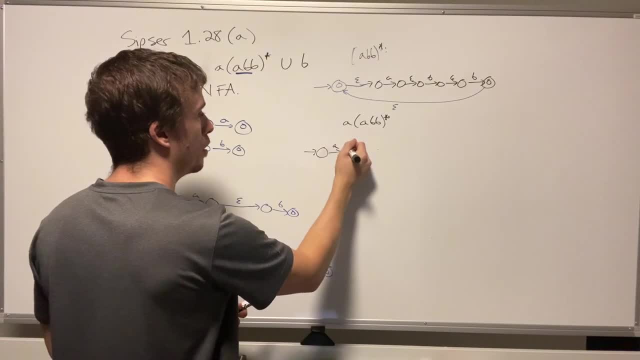 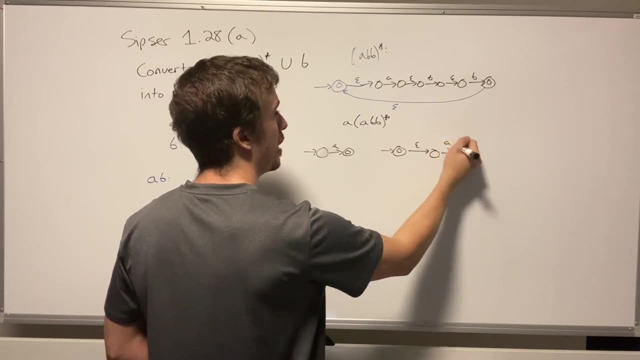 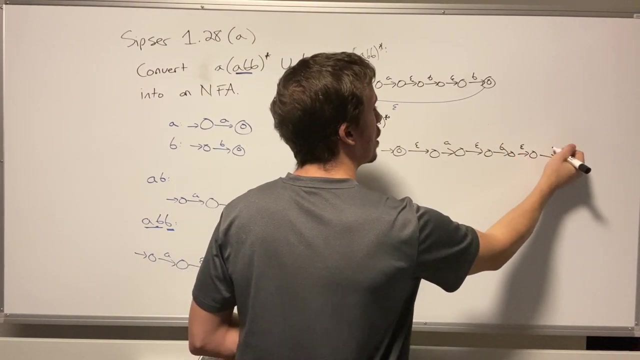 I should have made the state a little bigger. So there's the A thing, And then now I need the this thing. So this: there's an A epsilon, B epsilon. You can see why a computer is really good for the tool like this. 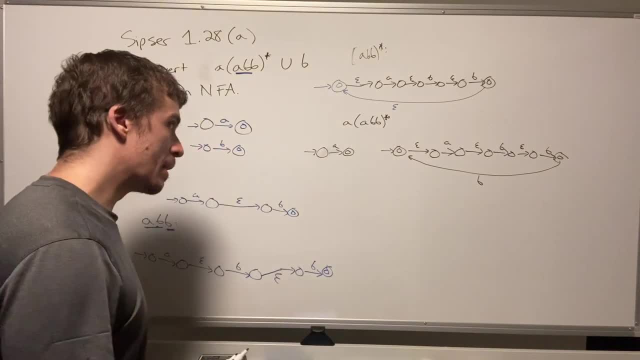 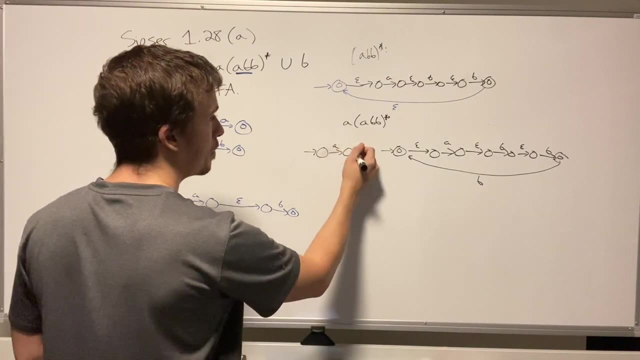 So there's that. So then, now we need to connect every final state from the first half to the start state of the second half, just like we did before. So, and with an epsilon transition. Actually, I'll put it above so it matches: 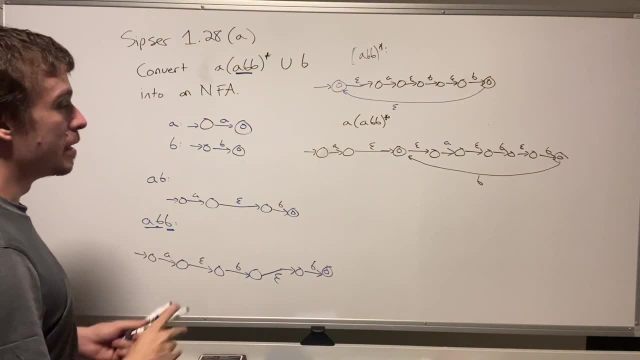 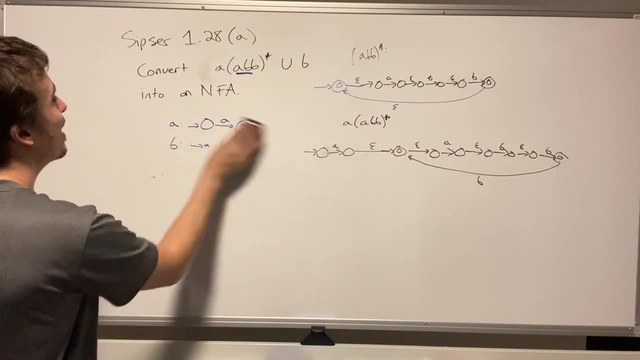 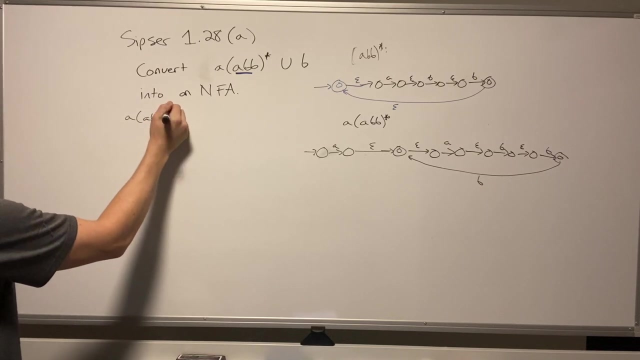 All right, So there we go. So then, now we did the first half. Now we just need to complete the whole thing. So I'm going to erase this, because this is going to be a rather big machine, All right, So then, let's, let's do this. So: A, A, B, B star, Draw the star a little better. 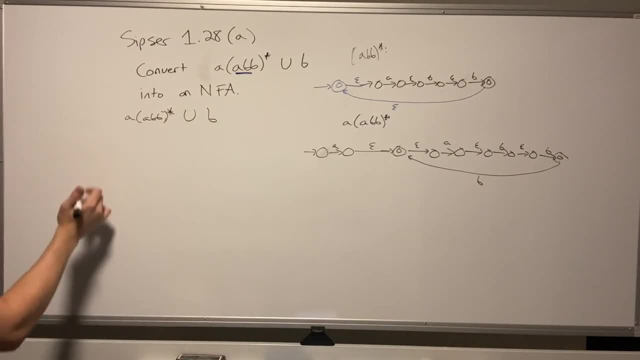 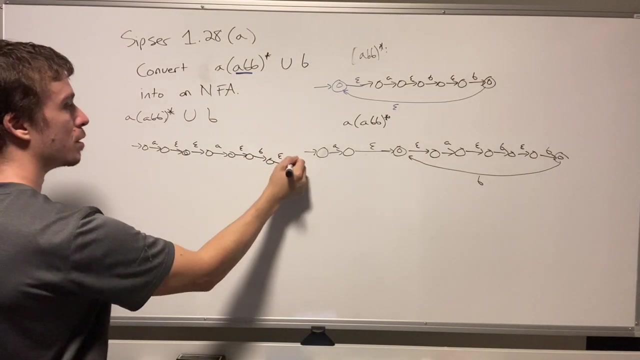 Union B. So then I'm going to copy that monster down, And for union we do things a little differently, where we arrange them on top, although you don't have to do that. So I'm going to have A epsilon- epsilon, So this one was a final guy, And then A epsilon B, epsilon B, And then this went back. 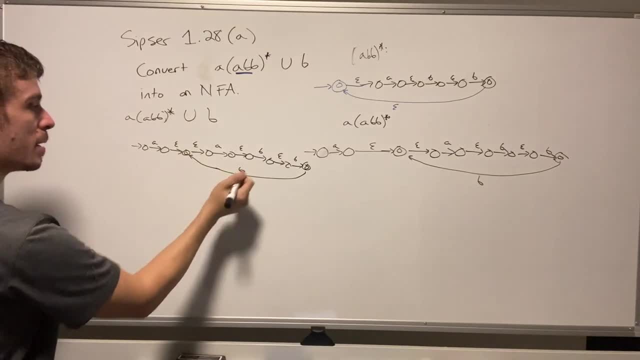 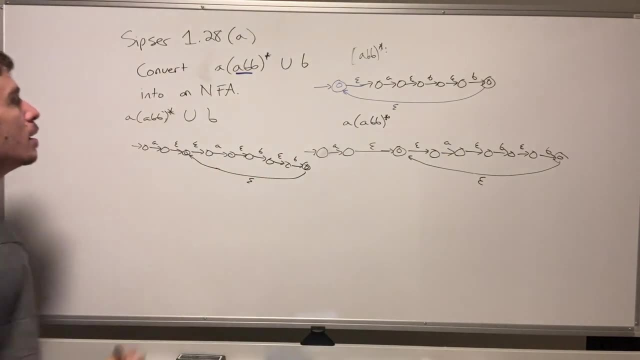 to here on B. Oh, I should have corrected myself. That's epsilon. I was wondering, why is it a B? All right, And then. so that's the first half. Now the second half. I'm just going to have B here. 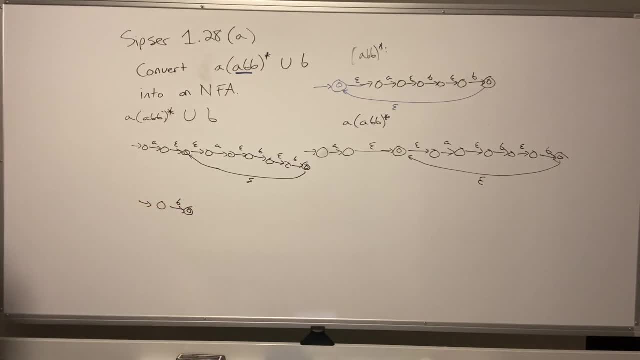 Okay, So then now what we need to do is to make a new start state that epsilon transitions to both of the original starting states. So I'm going to have a new one here. It's not going to be final, because we don't know in general whether or not the two halves are going to accept the empty string. 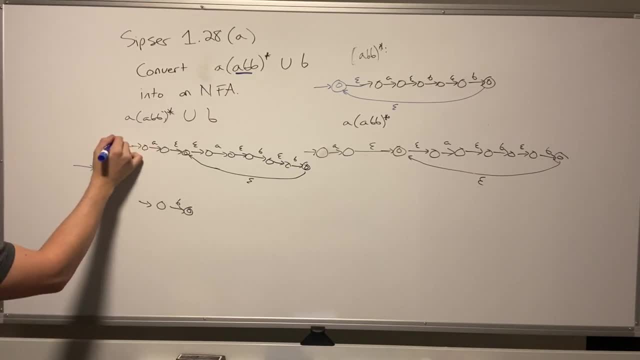 although it won't matter because we are doing epsilon transitions in any way. So even if one has the empty string, then we can just epsilon to that state anyway. So it doesn't matter And that's the corresponding NFA for that particular regex. So the procedure is extremely. 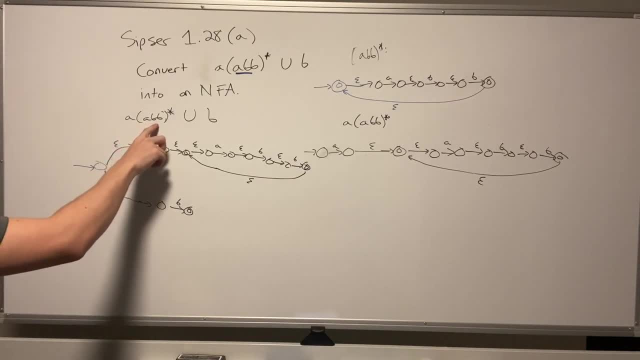 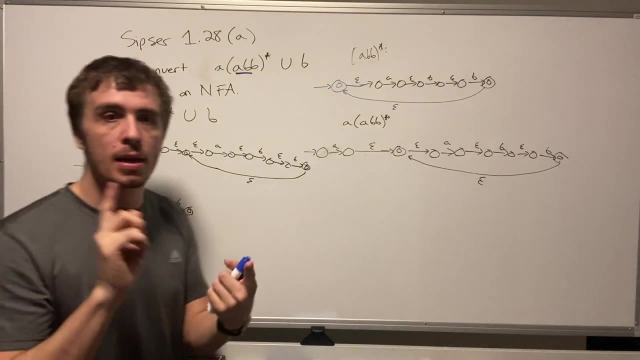 easy. All you have to do is to figure out each of the small components, things that can't be divided into smaller things, So ones that are not shown here are the empty string and the empty set- And you just make similar NFAs for those We did. 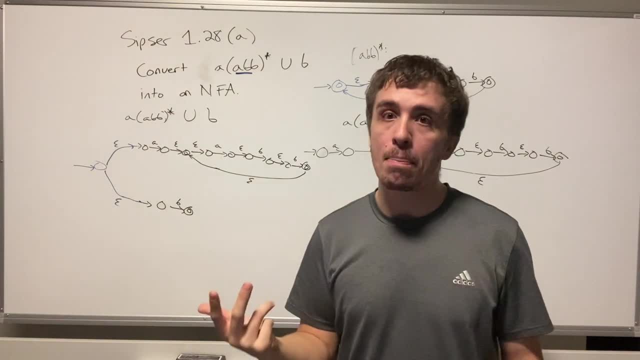 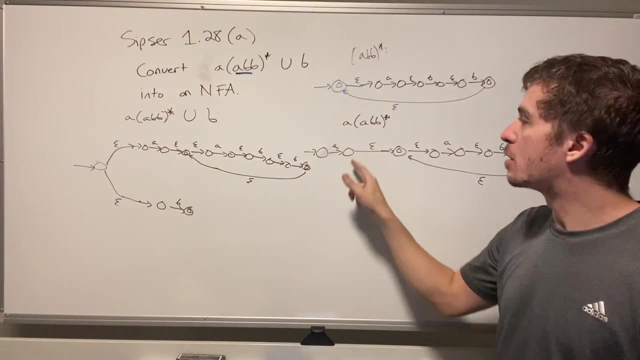 remove the ones for single letters, which are A and B, and the three operations are going to be concatenation, union and star. So concatenation, the whole idea is that every single final state of the first one, you epsilon, transition to the start state of the second one and make sure that 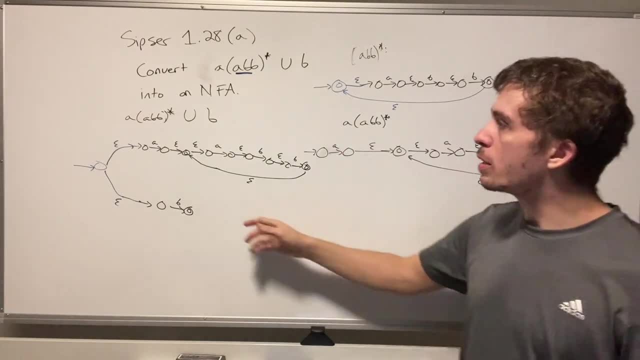 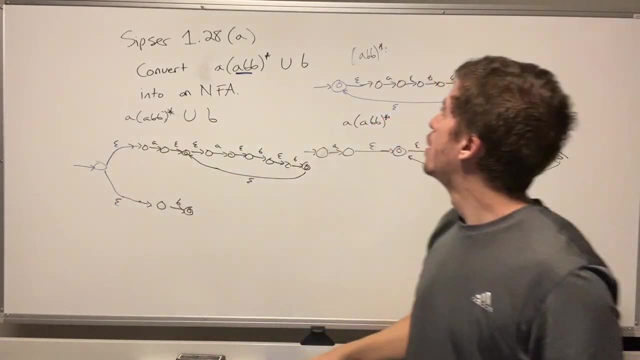 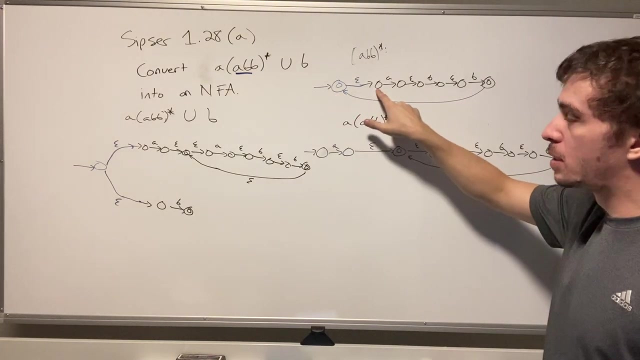 they're not final. on the left side, For union, you put the two machines one on top of each other, make a new start, state that epsilon transitions to both. And for star, all that you do is you put the original NFA down, make a new start. state that is final. epsilon transition into the old start state. 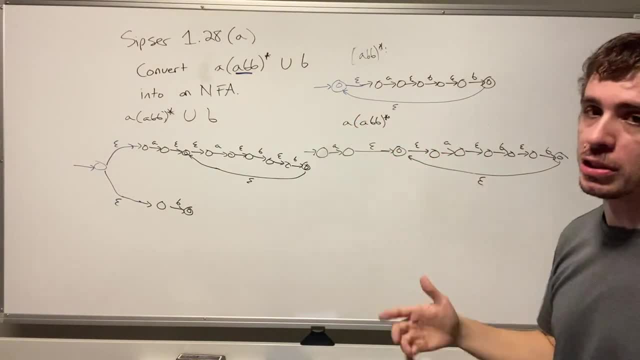 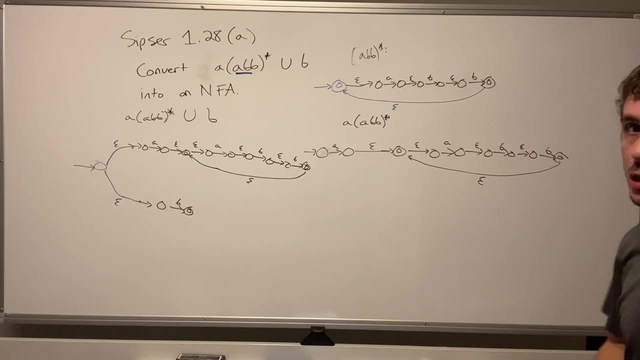 and epsilon transition either to the new one or the new old start state- It doesn't actually matter there. And this epsilon transition comes from every one of the final states in the original machine And that's how you convert any regex into an NFA. So hopefully that was interesting. 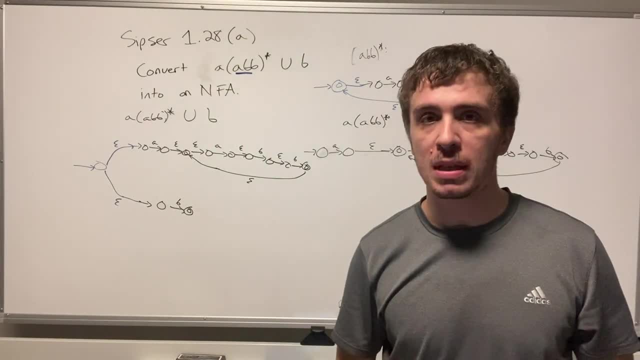 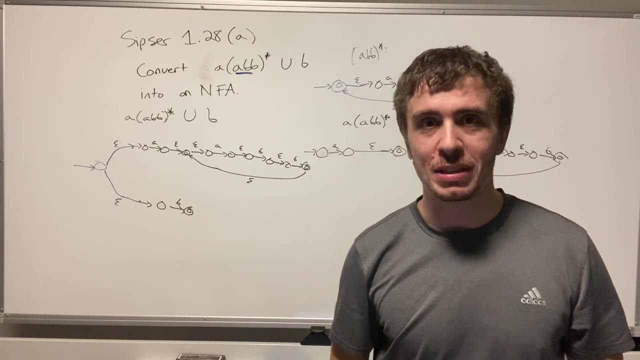 Leave thoughts about this conversion into the comments down below. As always, please like the video and subscribe to the channel. It really helps us out Any other links in the video description if you want to support the channel further. And, as always, thanks for watching and I'll see you next time. 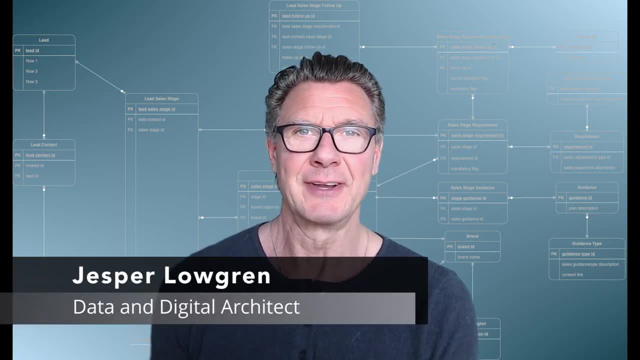 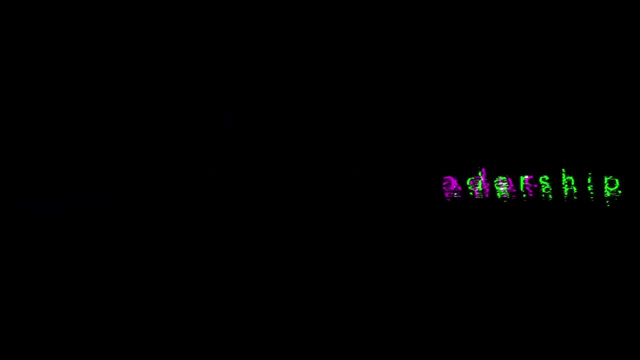 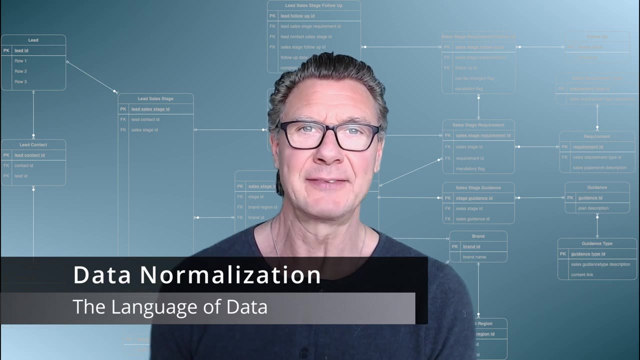 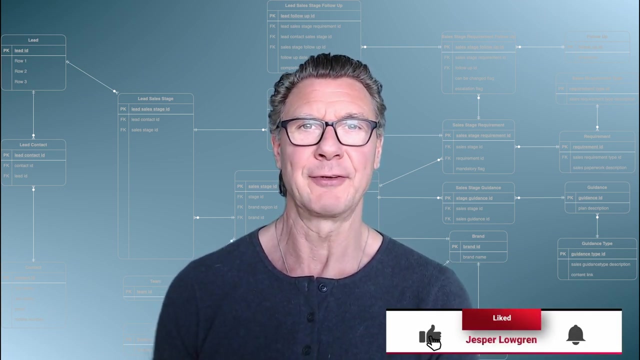 Hi, it's Jesper here. I make data architecture and digital transformation videos on YouTube. Today, I'm going to unpack data normalization, the language of data. Data normalization is both mathematics and philosophy, and I think you will get a sense for this as the video progresses. 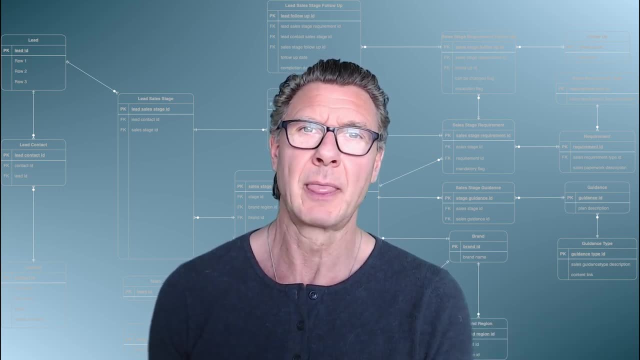 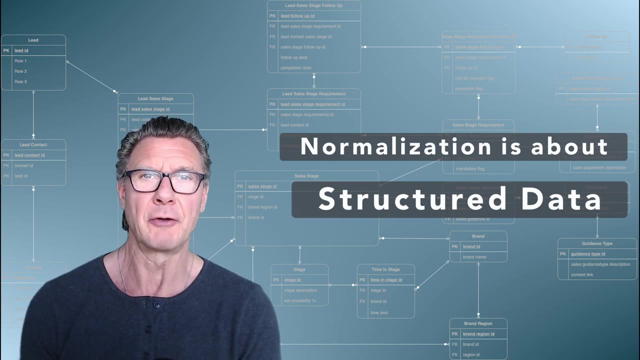 It doesn't explain everything, but it gives us a deeper understanding of one particular kind of data, which is called structured data, and how to connect structured data and do more with it, such as automation, analytics, prediction, artificial intelligence- all those fun and. 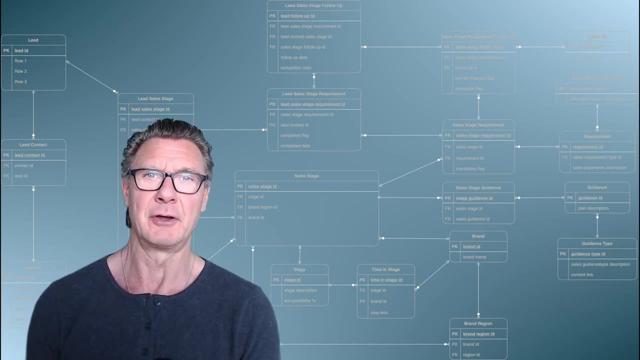 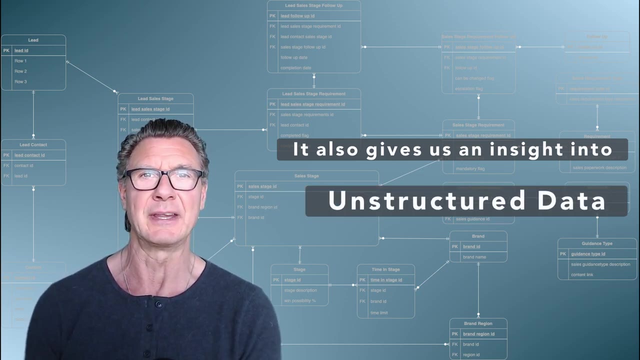 good things And, coincidentally or perhaps not, it also gives us an insight into the other side of data: unstructured data, the things that sit in spreadsheets, the things that are being generated, the things that are being used, the things that are being used, the things that are.